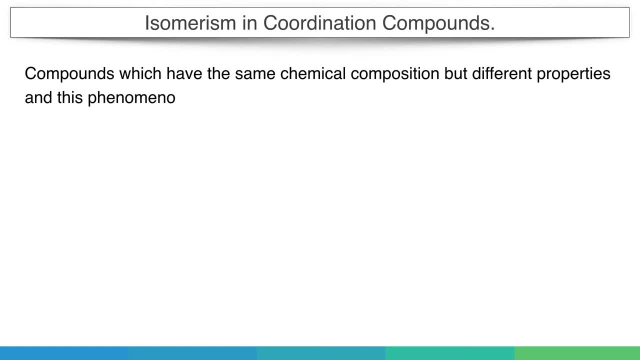 but different properties, and the phenomena is called as isomerism. The difference in their properties are due to different structural arrangements of their atoms. Though the phenomena of isomerism is very common with organic compounds, it is also found among inorganic compounds, particularly in coordination compounds. The various molecular arrangements which are 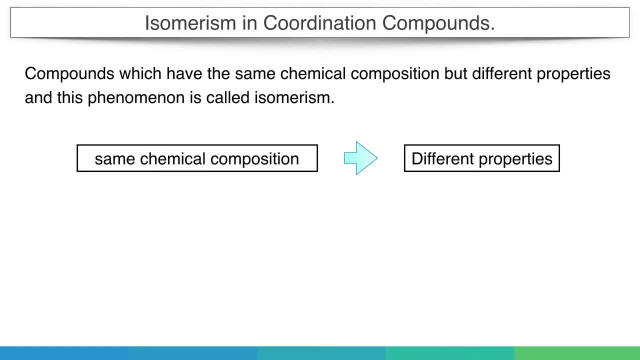 possible in coordination compounds produces more type of isomerism than are possible in organic molecules. There are three main types of isomerism Shown by complex compounds. They are: structural isomerism, geometrical isomerism, optical isomerism. Geometrical isomerism is also known as stereo isomerism. 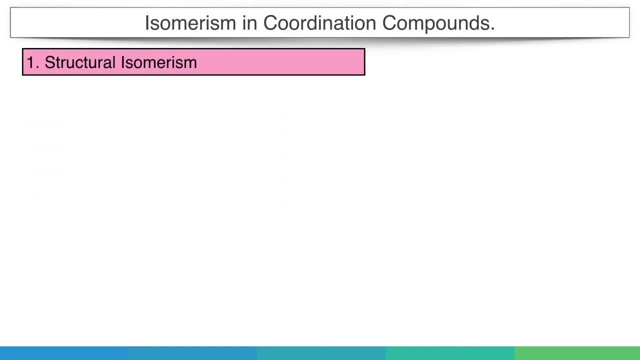 So let's take the first one: structural isomerism. As the name suggests, they will have different structures, Like here we show you two compounds. One is having bromine inside the square bracket and the other is bromine inside the square bracket. As you can see, these two molecules are having all the elements same, but only one group is inside. 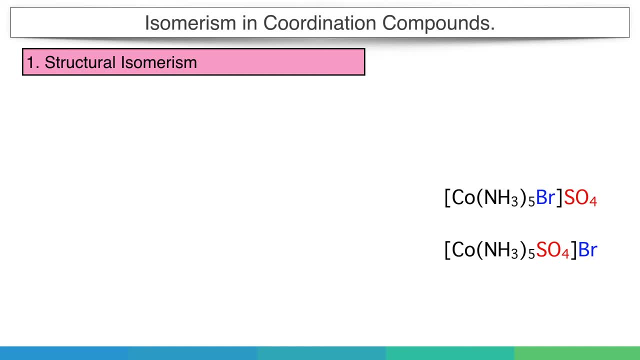 and other group is outside the square bracket. As we know, the ligands inside the square bracket are bonded with coordination bond and outside the square bracket by ionic bonds. This change of group will completely change the properties of two compounds, So these two are having same chemical. 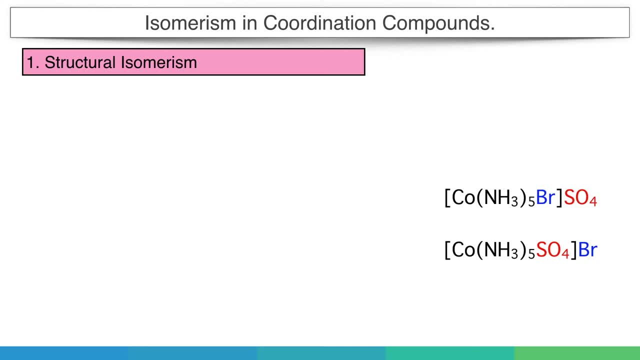 composition but different structures, So they can be considered as structural isomers. Therefore we can say that compounds which have same chemical composition but different structural arrangements are called as structural isomers. Structural isomers are further divided into five types: Ionization isomerism, hydrate or solvete isomerism, linkage isomerism. 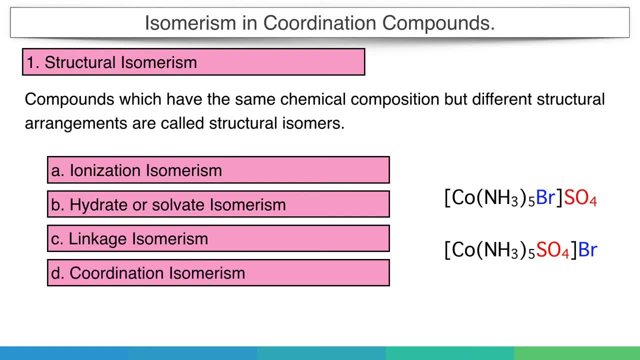 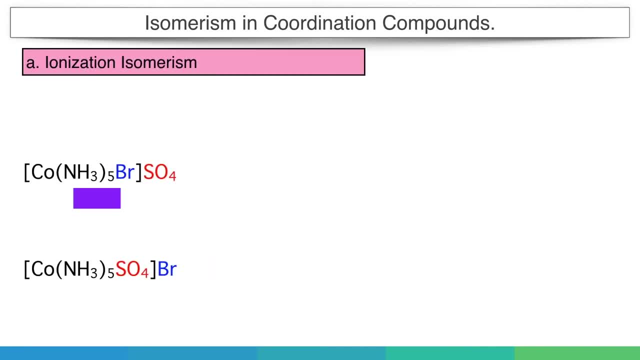 coordination isomerism and coordination position isomerism. Let's discuss all one by one. So first is ionization isomerism. As the name suggests, they are different in terms of ions. Let's take the same example as we discussed previously. So the first compound on dissociation. 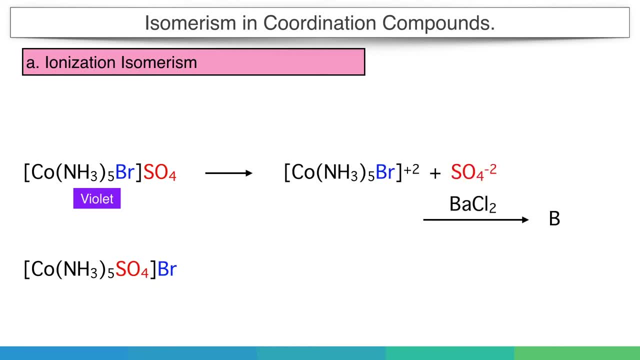 gives a complex ion and sulfate ion. There is no bromide ion formed in solution, but the second compound on dissociation gives bromide ion with a different complex ion. So in both compounds even they have both bromide and sulfate groups or they have same chemical composition. 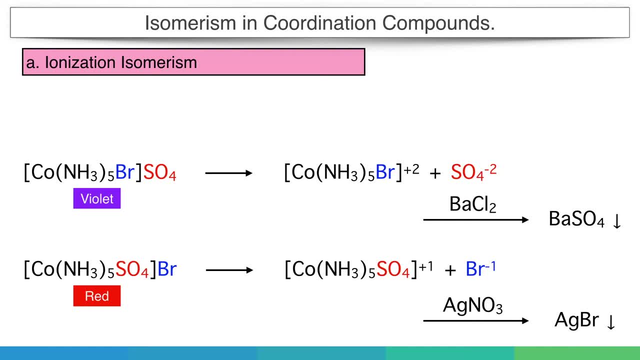 but on ionization or dissociation they produce different ions. One gives sulfate and other gives bromide ion. Therefore they are considered as ionization isomers. So we can say that compounds with the same chemical composition But forming different ions in a solution are called ionization isomers. Second comes 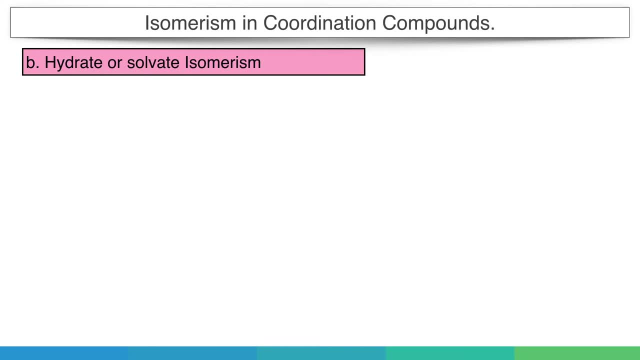 hydrate or solvete isomers. Some of compounds, when they crystallize, the empty space in crystal are filled with water molecules. This water molecule attached with the compound is known as water of crystallization And the compound is known as hydrated molecule. 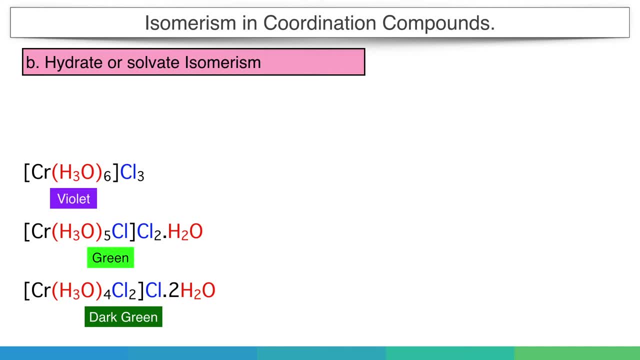 This water of crystallization is really rich in hydrogen and sodium. The hydrogen is available, is represented with the molecule after a dot. As water is also a ligand, it can form coordinate bond with the central metal atom. So even if the chemical composition is same, the water 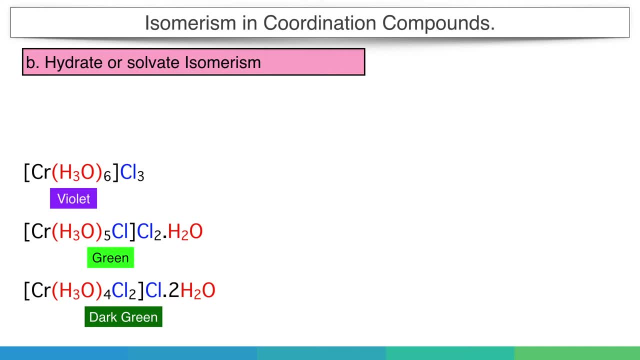 molecule can act differently. Thus this type of isomerism, where water of crystallization is different, is called hydrate isomerism. For example, here three compounds are shown which have same number of chlorine and water groups attached, But in first case all water molecules are bonded with coordination bond, while in second 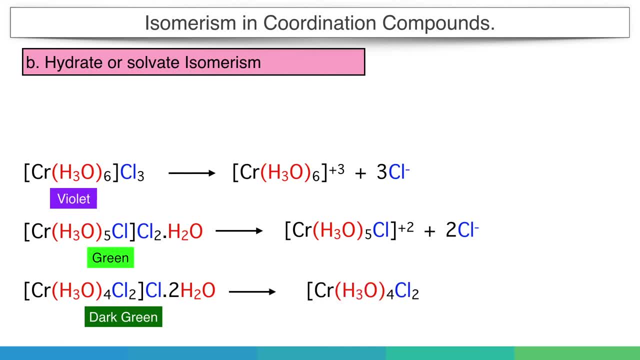 case one: water molecule is water of crystallization. It is not bonded to molecule. Similarly, in third case two, water of crystallizations are present. So when it is dissolved in water they only produce chloride ion as water of crystallization. 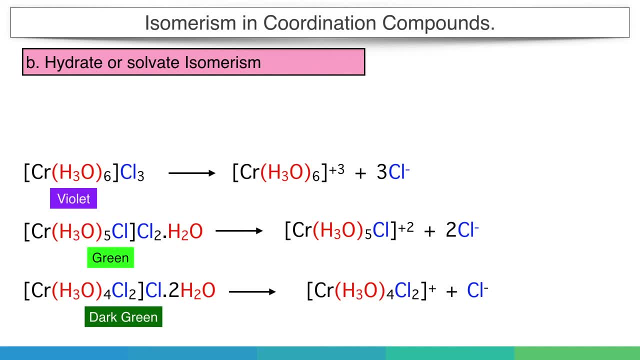 goes away. It is only present in crystalline form. but as you can see here, the number of chlorine ions liberated are different. that means they will show different properties. So compounds having the same chemical composition but differing in number of water molecule in the coordination sphere. 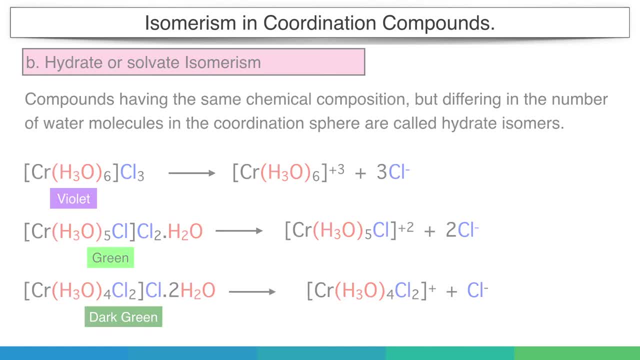 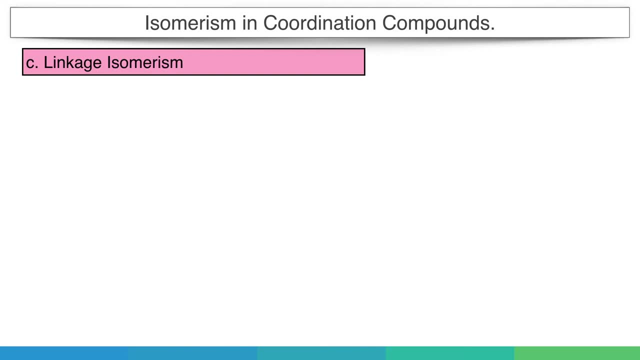 are called hydrate isomers. Next comes linkage isomerism. In the previous video, while explaining the types of ligands, we have discussed about the ambidented ligands. These are the groups which have two or more points of attachment, So they can attach to central metal atom from. 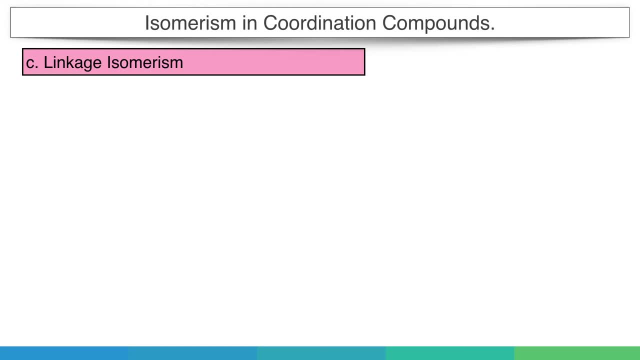 two different sides. So as the attachment changes, the properties of the bond changes And also properties of compound changes. Let's take one very common example of nitro group, In this case nitrogen and oxygen. both are having lone pair of electrons, So they can easily donate. 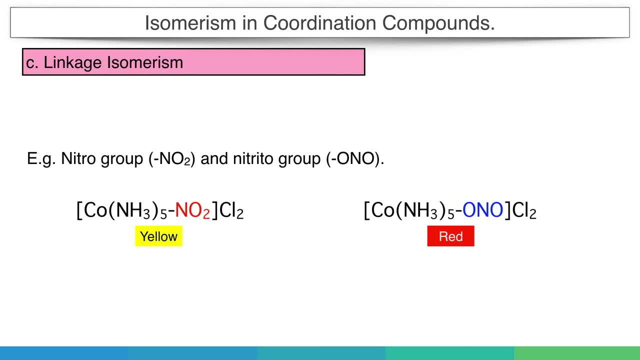 this lone pair and form a coordinate bond. When nitrogen donates one lone pair, the group becomes nitro group, and when oxygen donates the lone pair, it becomes nitrito group, As in case of nitro penta amine, cobalt 3 chloride, which is yellow in color, and nitrito penta amine. 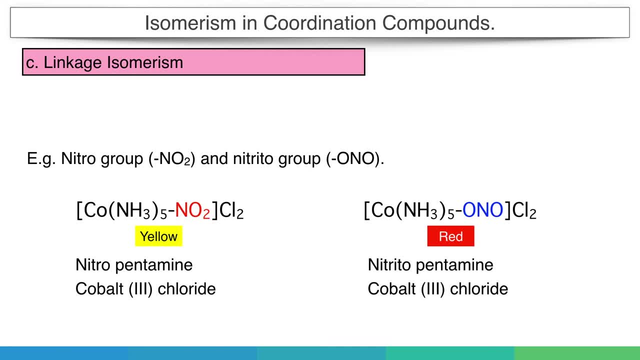 cobalt 3 chloride, which is red in color. So they have same chemical formula but different properties because of different point of attachment. So we can say that compounds having the same molecular composition but different mode of attachment of ligand to the metal, These compounds are called as linkage isomers. 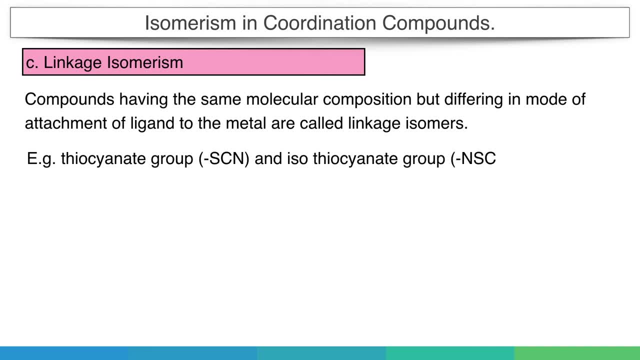 Another example of same type is thiosinate group, Which have sulfur and nitrogen as donor atoms. Sоль. wann sulfur slides, tastes alone pair, it becomes thiosinate group. and when nitrogen donates lone pair, it becomes a isothiocinate group. Next comes coordination: isomerism: Complex compounds can have both the ions positive. 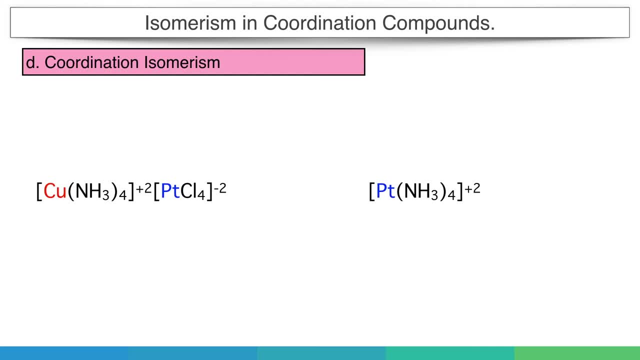 and negative as complex ions. This means none of them is normal ion, but they both are complexes. In this case, if the ligands are interchanged from the positive ion to negative ion or vice versa, the chemical composition remains the same, but as the complex ions are now different, they will show different. 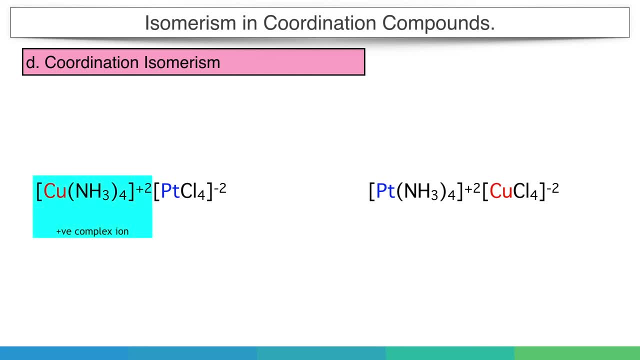 properties. For example, here are two compounds with positive and negative complex ions. Both sides are kept in the square bracket. That means both are coordination compounds and none of them is simple ion. Now, both compounds have same chemical composition, but in first case ammonia ligand is attached to copper and in second compound, ammonia is attached to. 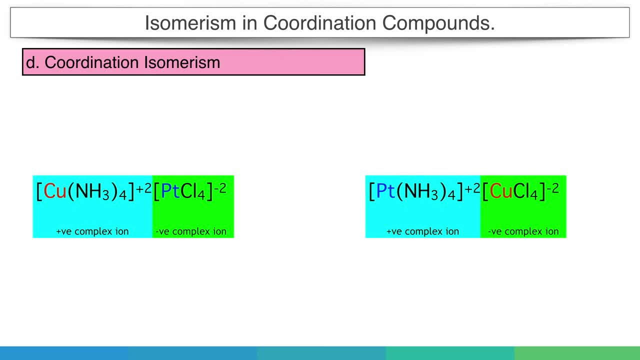 to platinum. similarly, in first compound chloride is attached to platinum, but later it is attached to copper. so even their chemical composition is same, but they will show different properties, as the complex ions are now different, or we can say the ligand are coordinated differently. so as per the definition compounds where both cations and anions are complex ions, the distribution: 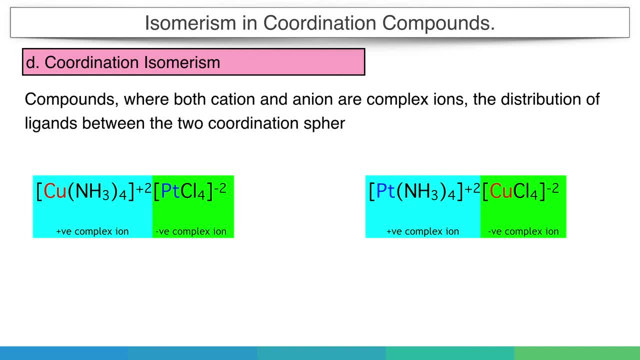 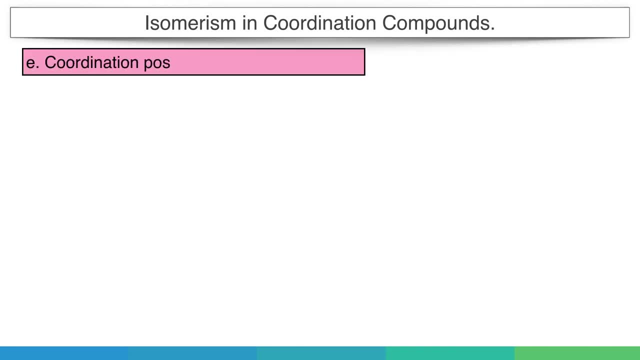 of ligands between the two coordination spheres can vary and give rise to coordination isomers and finally, coordination position isomerism. in simple words, we can say that the ligands are coordinated at different positions. for example, in the given compounds there are two cobalt atoms and in one case both cobalt atoms are coordinated with three. 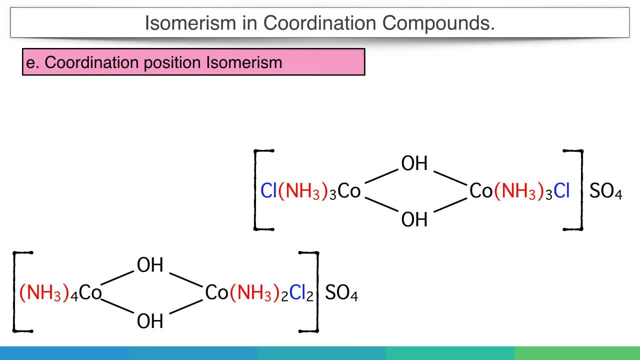 ammonia and one chloride ligand. but in other compound one cobalt is linked with four ammonia ligands, while second cobalt is linked with two ammonia and two chloride ions. so the position of coordination of ligands changes from first cobalt atom to second cobalt atom. 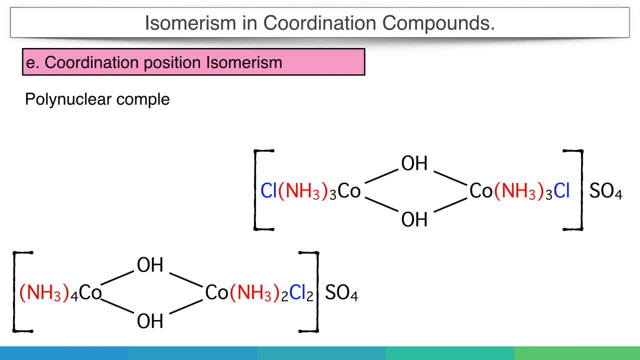 Therefore we can say that polynuclear complex compounds having the same number of coordinating groups that are distributed in different ways around the metal ion are called coordination position isomers. So that was all about the structural isomerism and it is possible that